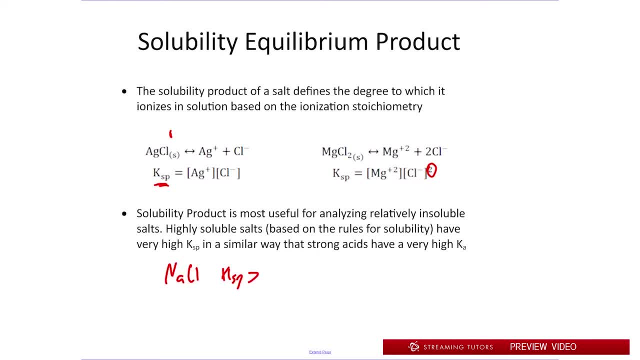 the very soluble salt. its Ksp is just going to be extremely large, way greater than 1.. In general for the typically insoluble salts, you'll remember that from general chemistry 1,, when we went over the rules of solubility For generally insoluble salts, Ksp is much. 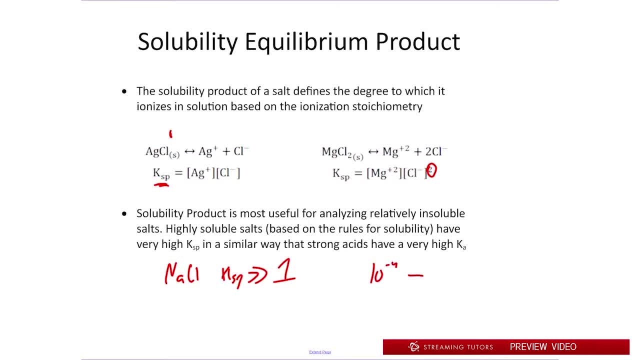 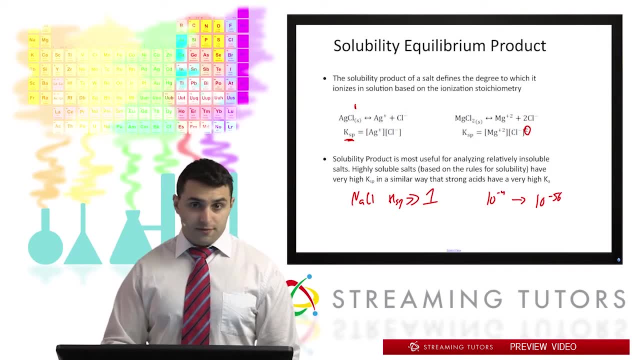 smaller, something between anywhere from 10 to the negative, 4 to 10 to the negative 56,. what have you? So? Ksp is going to be most useful for looking at relatively insoluble salts and seeing what amount of ions are formed by them in. 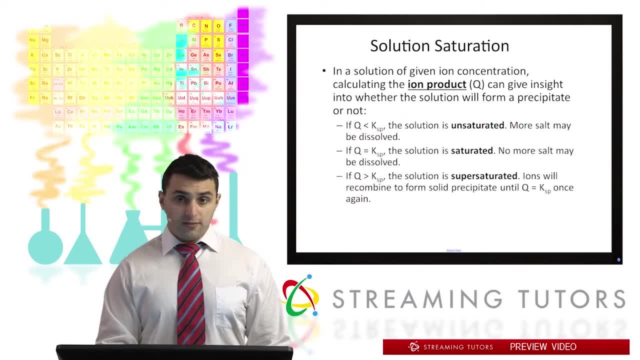 solution. One other thing we can talk about, based on Ksp, is the saturation of a solution, And we're going to use the ion product Q once again to look at whether a solution can dissolve more ions can is fully saturated or whether it will form a precipitate. So 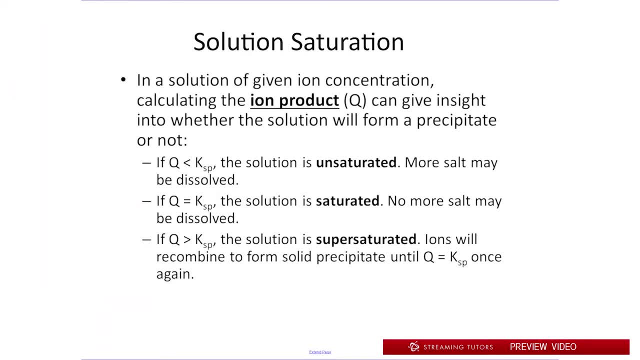 in general, the way that it's going to work is as follows. So if our ion product is less than Ksp, that means the solution is unsaturated and so more salt can be dissolved, meaning that equilibrium would shift to the right. If Q equals Ksp, that means we have 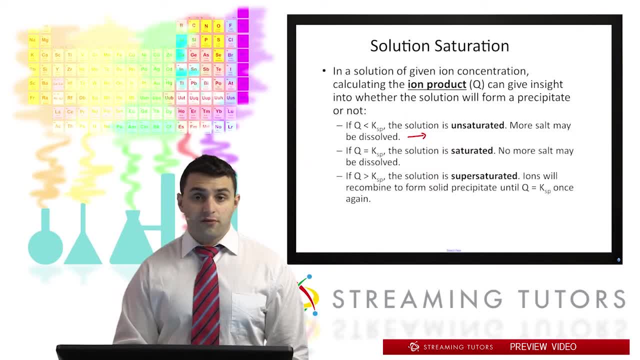 a fully saturated solution, meaning that we can't dissolve any more of the salt. And dissolving any more is not going to dissolve the salt, it's just going to stay there as a precipitate. So that's when Q equals Ksp, that's known as a saturated solution When Q is greater. 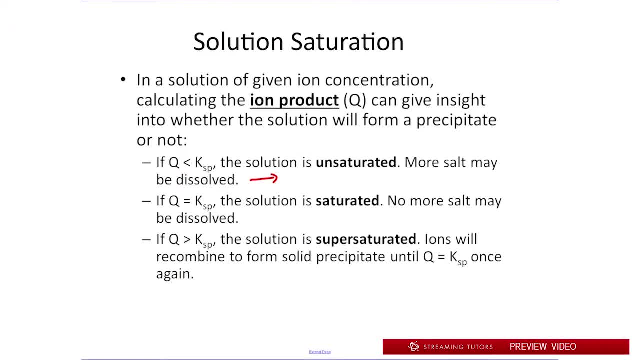 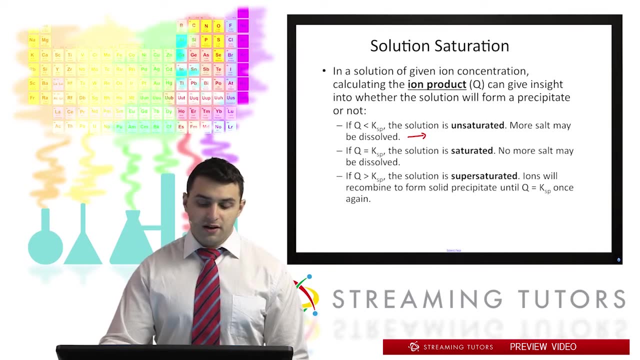 than Ksp. that's when we have a supersaturated solution. So when that happens, we have too much salt dissolved in the solution, so that not all of it can be dissolved. What will happen then is that ions will recombine to form the precipitate or the solid salt, until 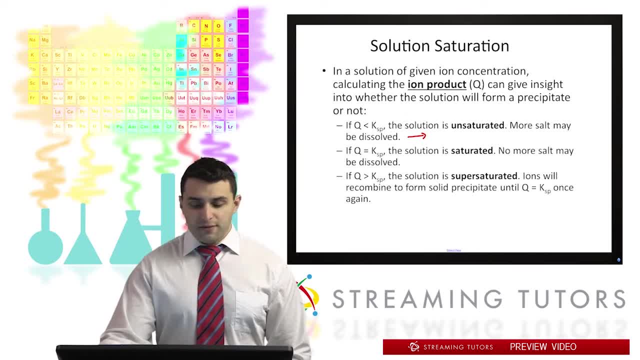 Q equals Ksp once again. So the basic premise to get away from this, that's shifting equilibrium to the left, just like it was in the first example. The basic thing to take away from this is that there's a set limit on the solubility of a salt in a given set of conditions, whether 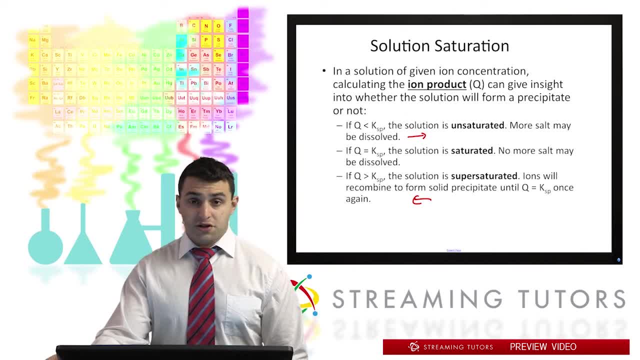 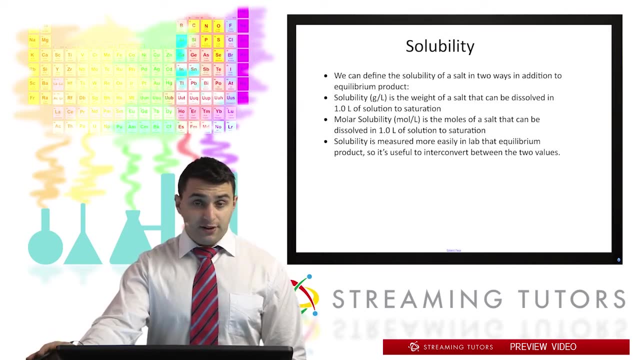 that be, in water at a certain temperature or in a certain concentration of another salt or an acid base. what have you So? what we can do, then, is we can be given a concentration of a salt added and we can see whether- okay, is this going to be enough salt to dissolve? 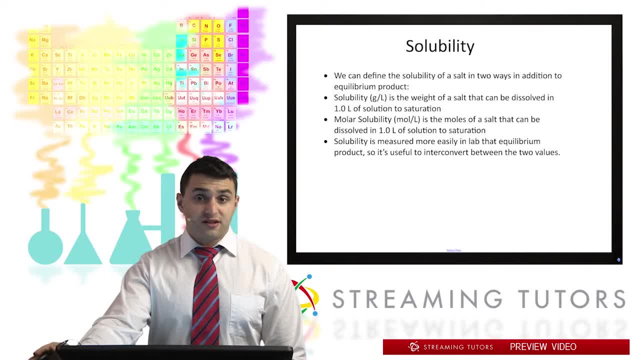 to form precipitate, is there going to be not enough added to saturate the solution, and so on. So the way we typically look at Ksp in a solution is by looking at the solubility. So there's two common ways we can define solubility. The first is just normal old solubility, That's. 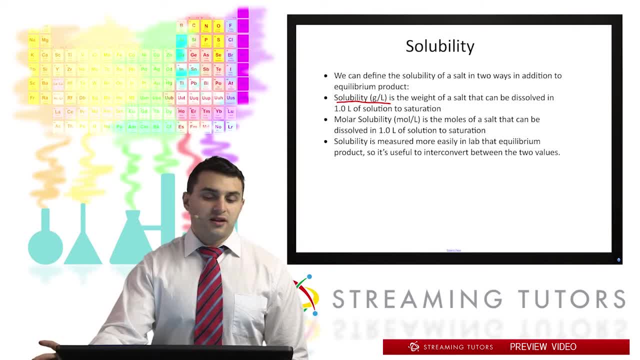 in grams per liter. So that's saying what is the weight of salt that can be dissolved in a one liter solution. It's the weight of the solution until the point of saturation. The other way to do this is through molar solubility, which is just saying the same thing in terms of moles per 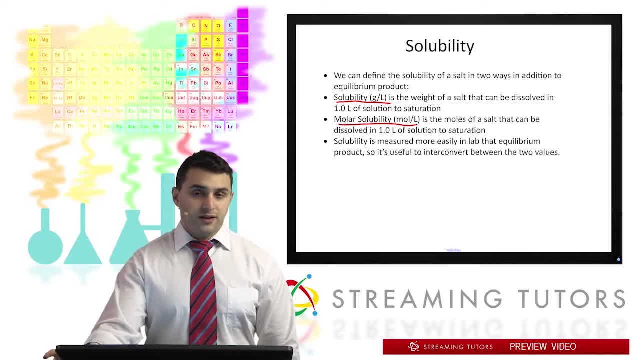 liter instead of grams per liter. So if you think about solubility, we can pretty easily determine how much of a salt we can dissolve in a certain amount of media. Obviously, as we keep adding more and more salt, eventually it'll just stop dissolving, So we can use. 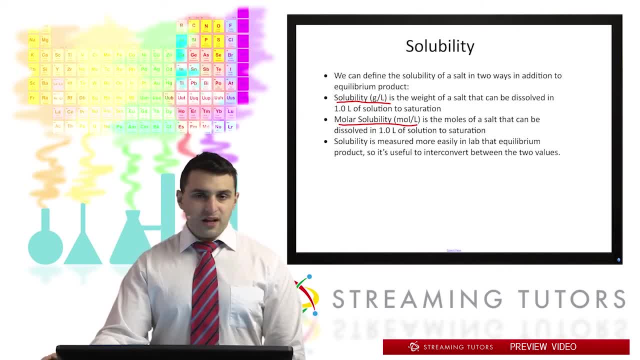 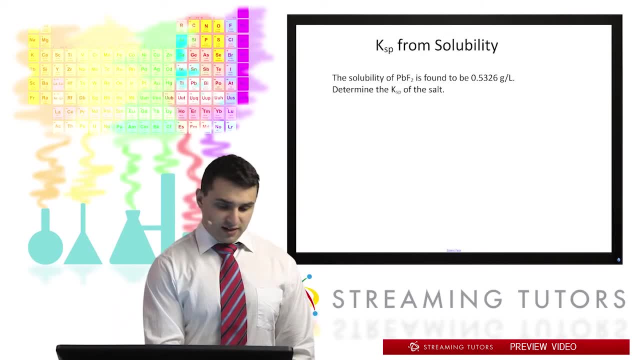 solubility to determine then the Ksp of a salt. and we can also do vice versa. So let's take a look at some examples of that. So in this first problem here we're told the solubility of Pbf2 is found to be. 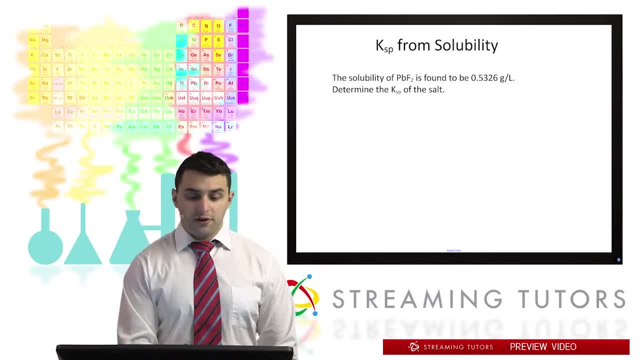 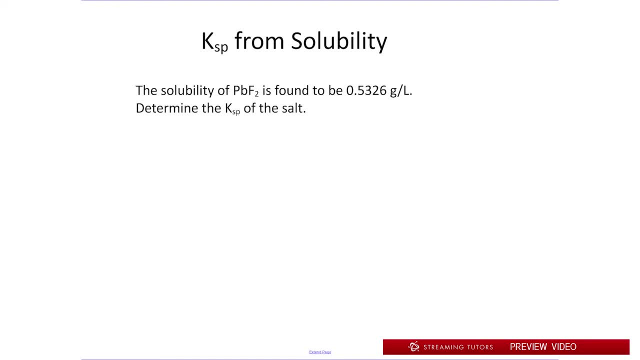 0.5326 grams per liter and we want to determine the Ksp for the salt. So the first thing we want to do is write an expression for the dissociation of Pbf2.. That'll look something like this. It'll look something like this: 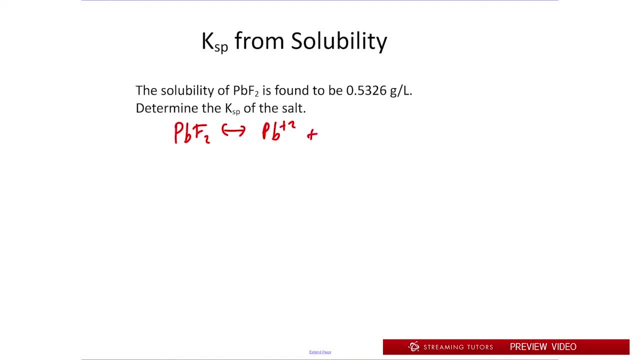 It'll look something like this. It'll look something like this: So I want to perform Pbf2 and two F- ions. Okay, So we have that expression then. So we can write then an expression for Ksp. We're gonna say that Ksp is going to be equal to. 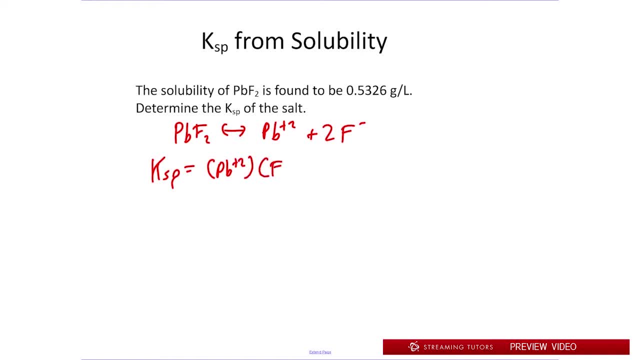 the concentration of Pbf2 times the concentration of F- and we're gonna square that because of the coefficient that we see in the dissociation. So the next thing to do, then, is we have to find a way to relate Ksp and the Ds. 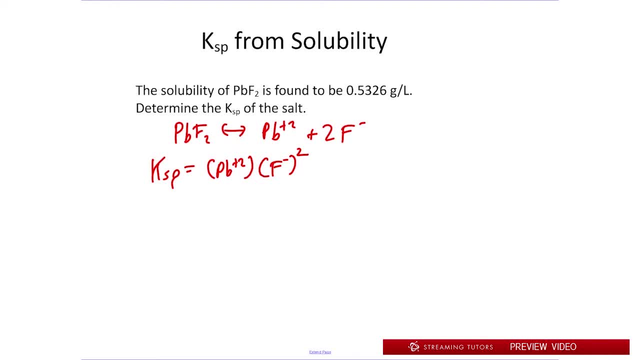 So the next thing to do, then, is we have to find a way to relate Ksp and the Ds. So the next thing to do, then, is we have to find a way to relate Ksp and the Ds, the ion concentrations. 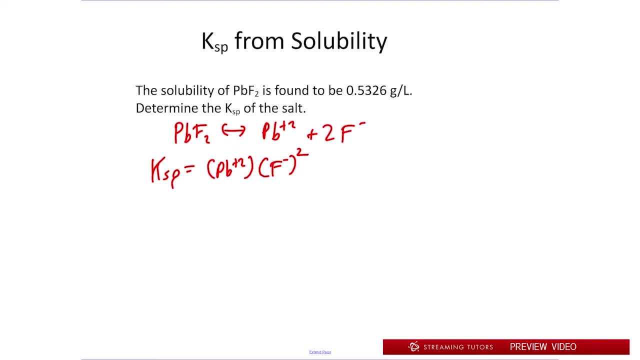 The way we're going to do, that is, we're going to say: we're gonna say that we can substitute the solubility of each of these ions in for its ion product. So what we can say, then, is: we can call the concentration of PD plus two S for solubility. 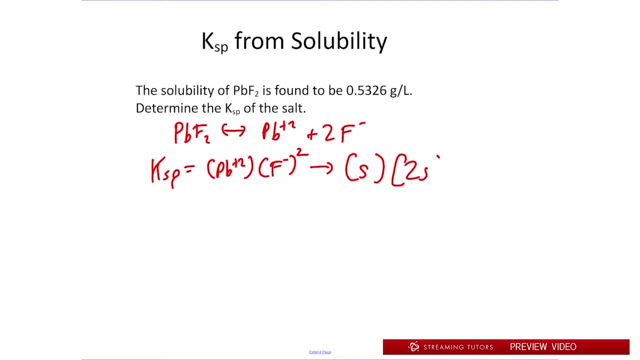 The concentration of F minus would be two S, since there's double the amount of fluoride. and then we have to square that term. So we're putting solubility in here, because the solubility is gonna determine the maximum amount of ions or the maximum amount of salt that can be dissolved. 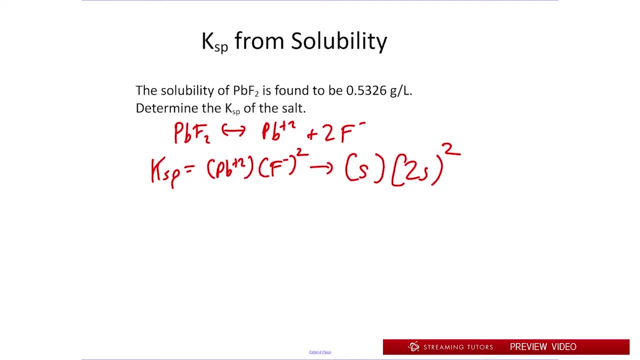 So that's obviously gonna be related to the solubility of the salt. Now, the one thing we have to remember here is that we're looking at concentrations. we have to do things in moles per liter molarity. So the other thing we have to do 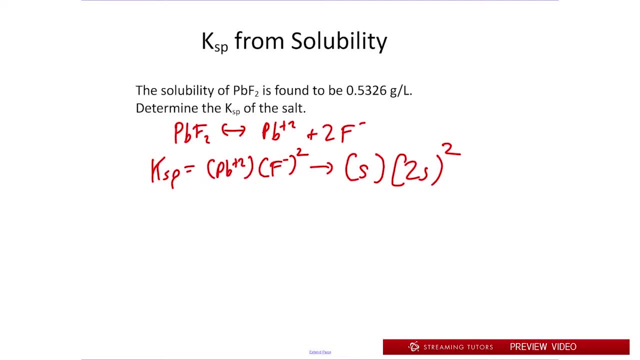 is we have to just convert from this solubility to a molar solubility. So if we have a solubility of 0.5326 grams per liter, we can convert that into moles per liter by just simply dividing by the molar mass of PBF2.. 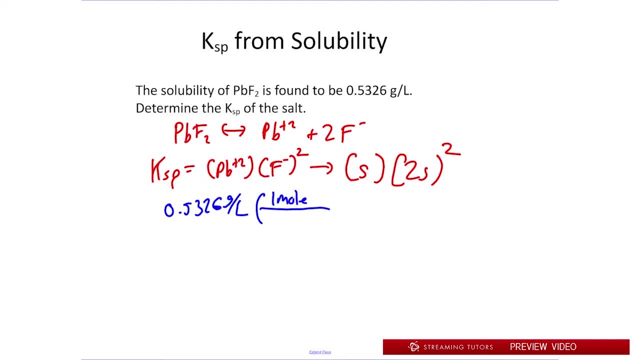 So that'll look like this: The molar mass is 245.2 grams, And so that gives us a molar solubility of 2.17 times 10 to the negative three, And that's in moles per liter. 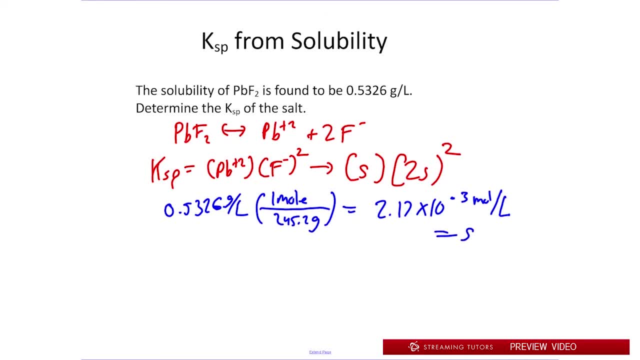 So what we can say, then, is that this is equal to the S that we're gonna plug in to determine our Ksp. So if we have that now, we know from here that our Ksp is simply gonna be equal to S times four S squared. 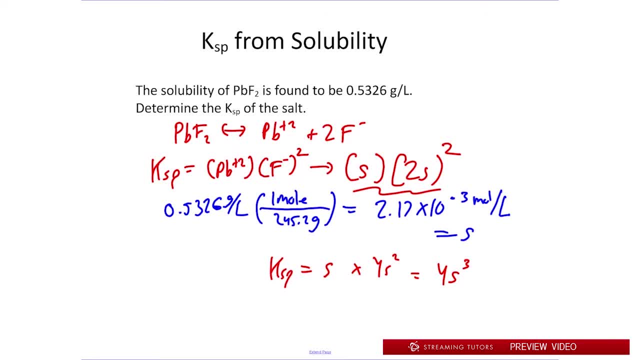 So that's gonna be equal to a total of four S cubed. And we found our solubility: our S is equal to four S cubed, And now all we have to do to find Ksp is to simply plug this value in.